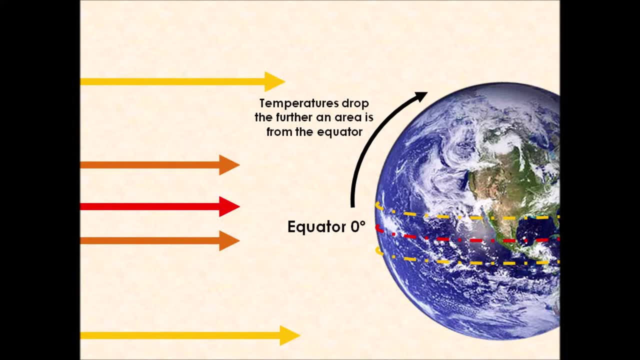 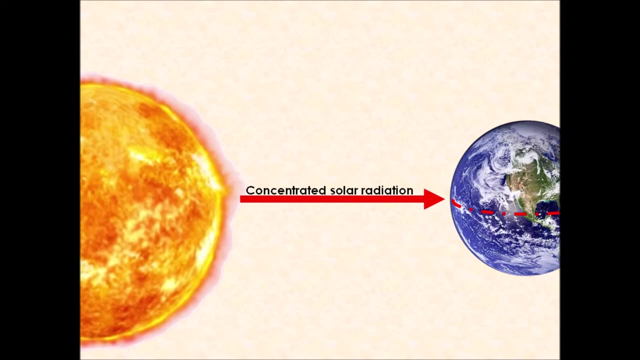 However, global atmospheric circulation is not the sole reason for these different climate zones. Latitude is probably the most important factor to influence variations in climate zones, due to the curvature of the surface of the earth. Now we know that the equator receives the most concentrated amount of solar radiation. 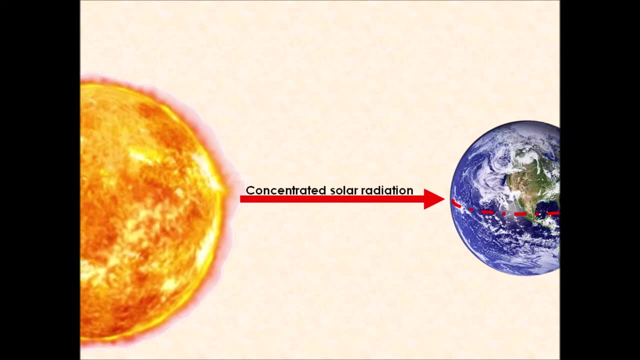 or sunlight compared to the north and south pole and, as a result, on the equator the air is heated more intensely and then it becomes less dense and lighter, causing it to rise to a higher altitude, which leads to evaporation taking place and cloud formation. This creates a global climate zone which 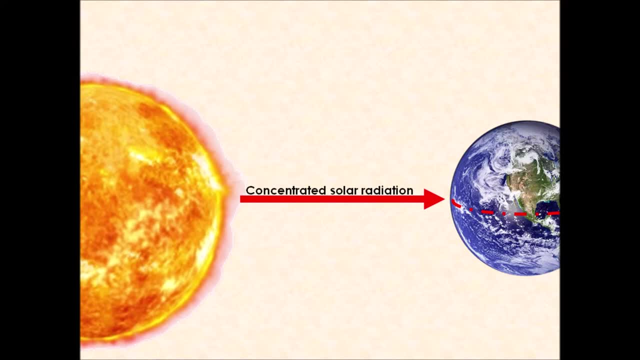 is known as a low pressure belt along the equatorial zone. so along the equator. Now, after rising, the air does spread out and begin to flow towards the north and south pole, and that is where your global atmospheric circulation concept comes in. So again, if you're not very confident, 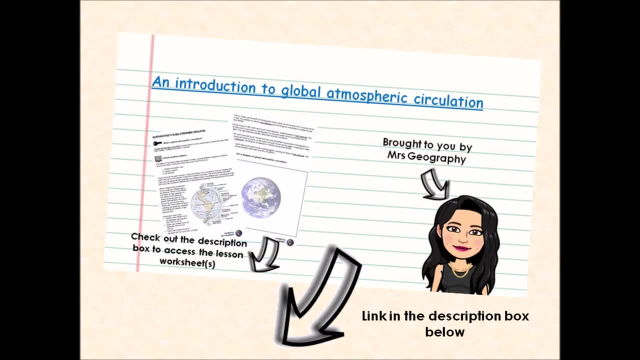 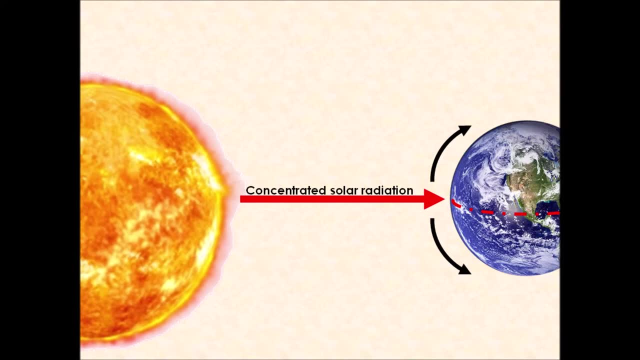 with global atmospheric circulation- check out my previous video- So as that air then spreads out and begins to flow towards the north and south pole, it then obviously will sink and descend and create high pressure. On the other hand, the polar regions, the very far north and south of our planet. 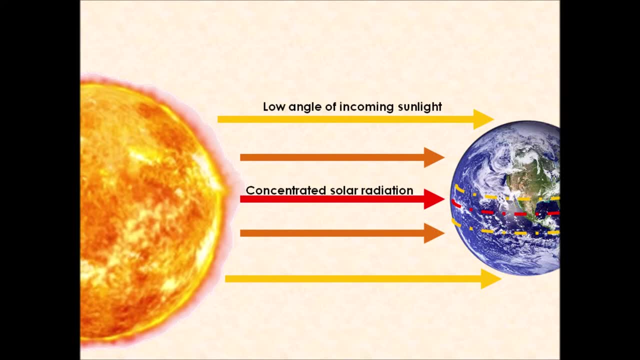 receives a less concentrated amount of solar radiation And sunlight, resulting in colder, dense air and high pressure. This is because, as the air sinks towards ground level, it spreads out and again then flows back to the equator. Now, together, the low pressure of the equator and the high pressure of the poles creates what we call convection cells. 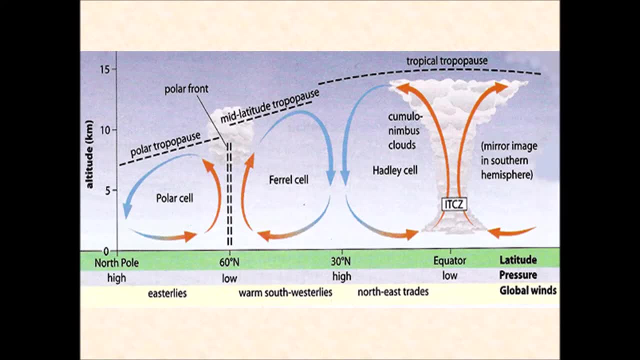 This links to the concept of global atmospheric circulation. So just very quickly to summarize what a convection cell is: It describes differences in air temperature leading to the formation of these high and low pressure areas, And these areas become linked together by the circulation or flow of this warm. 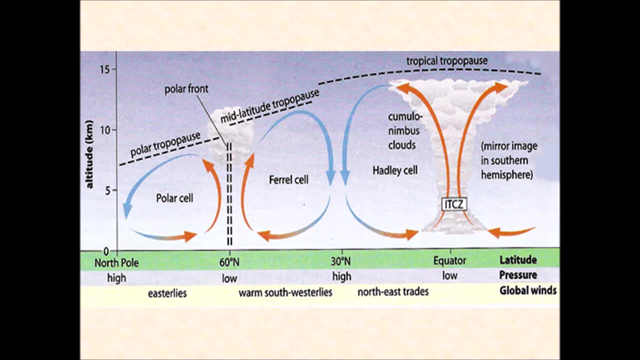 and cold air. So very quick diagram to summarize these convection cells. you can see on the screen now. So you can see on the equator we've got your intertropical convergence zone, your ITCZ, and this is where you have that rising air. 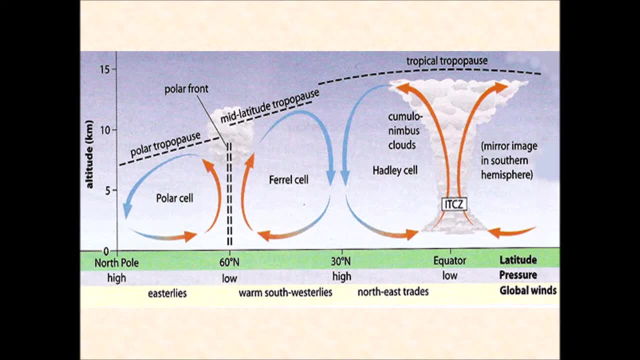 That then will travel from your equator towards your 30 degrees north and 30 degrees south within your Hadley cell. But at 30 degrees north that air is descending, it's sinking to create that high pressure at 30 degrees north And the air will then travel in one of two directions. It will stay. 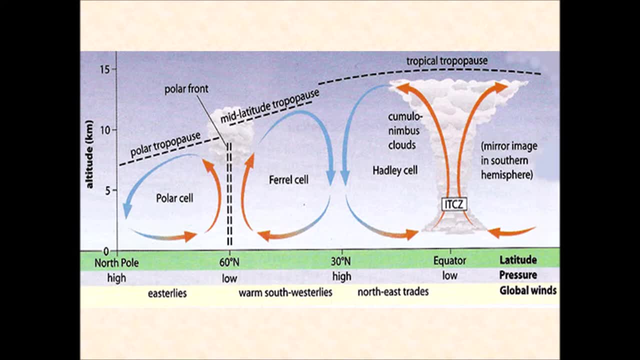 within the Hadley cell and circulate back to the equator, Or it will travel into the ferrule cell and it will then move from 30 degrees north to 30 degrees north, And then it will travel back to the 60 degrees north and south. At 60 degrees north and south it will then rise again, creating 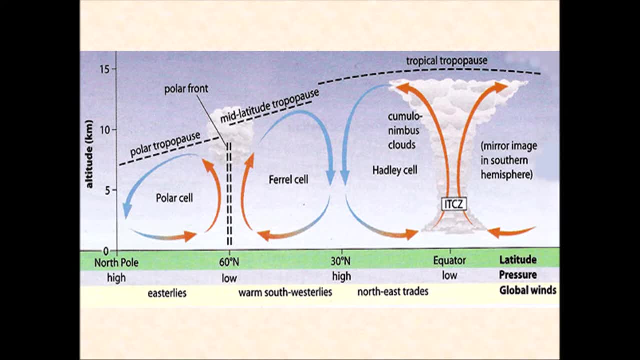 that low pressure because we've got condensation taking place high in the atmosphere, And then again it will circulate back round either into the ferrule cell or into the polar cell, And if it travels in the polar cell it will travel towards the north or south pole, creating 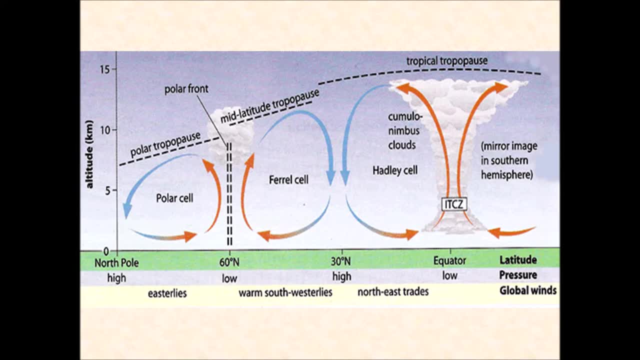 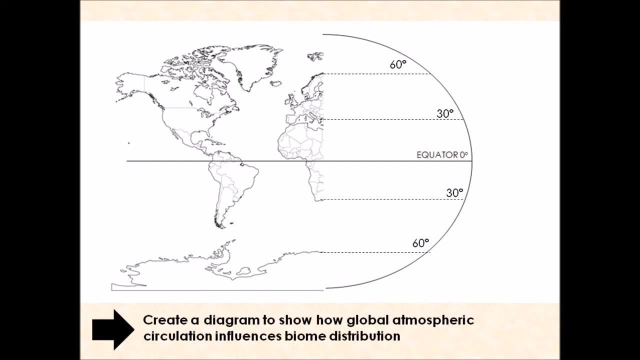 again that sinking air, that descending air leading to high pressure. So how does global atmospheric circulation influence climate zones or biome distribution? And this, obviously, is a lovely synoptic link to the topic of ecosystems, again studied in many GCSE specifications. So we're going to basically create a diagram to show how. 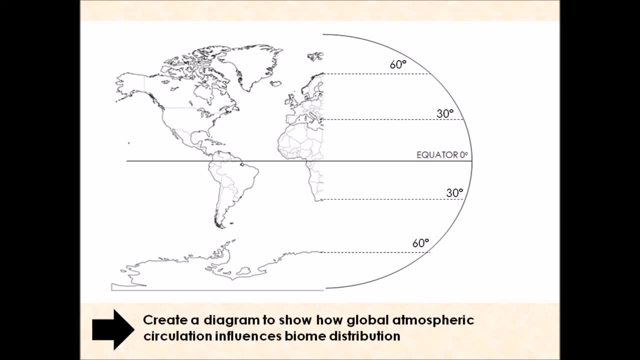 global atmospheric circulation influences the distribution of our biomes, our major biomes in the world, Our tropical rain forests, our deserts, our savannah and so on. So we're going to start off with a diagram, If you're working on the worksheet. 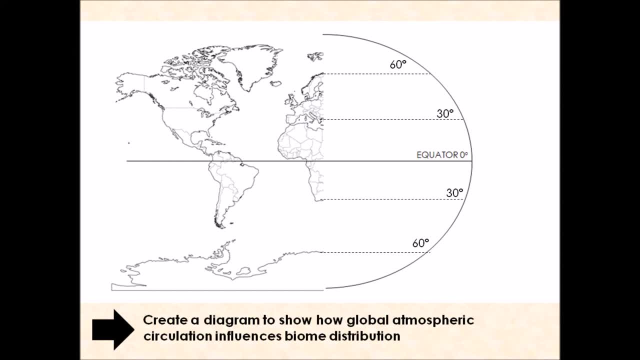 I've already prepped it for you. I'm basically going to add some more details in. If not, obviously you can attempt to draw this out. it's entirely up to you. So we're going to start off by putting our convection cells on there, linked to global atmospheric circulation. So we've got. 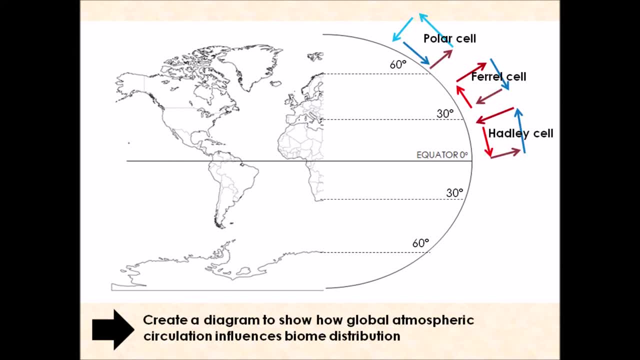 our Hadley cell, between zero degrees on the equator and 30 degrees north. Then we've got our ferrule cell, 30 degrees north to 60 degrees north, and then we've got our polar cell, which would be 60 degrees north to the north pole. Now I'm only going to focus on the northern hemisphere. 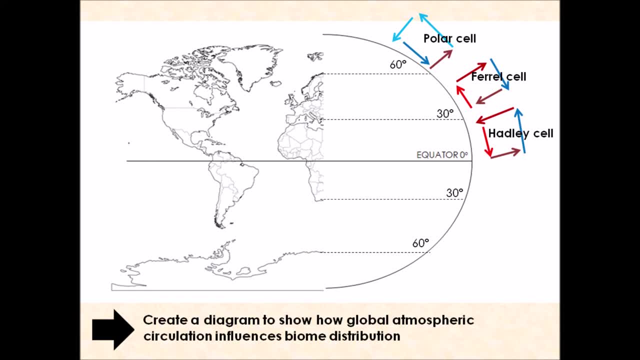 today, because it is a mirror image, if you like. So if we were to look at the lower half of the diagram, from your equator to 30 degrees south, you would have your Hadley cell. from 30 degrees south to 60 degrees south, you'd have your ferrule cell. and from 60 degrees south to the south pole, you'd 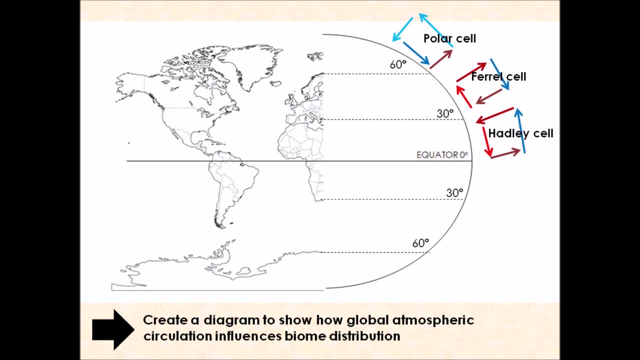 have your polar cell. But just to make sure your diagram doesn't look too busy, at the end we're going to just stick with our northern hemisphere and then, if you want to copy this out later as a mirror image, you're more than welcome to. So we've got our convection cells on there now. 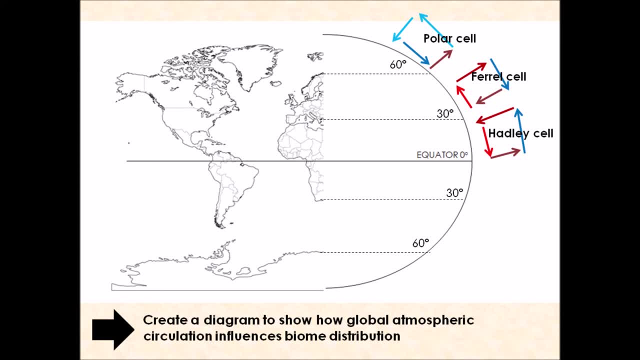 Now we're going to also add in those areas of high and low pressure. So on the equator we have got an area of low pressure because that air is rising, Whereas at 30 degrees north, between your ferrule and Hadley cell, you've got a h for high pressure. 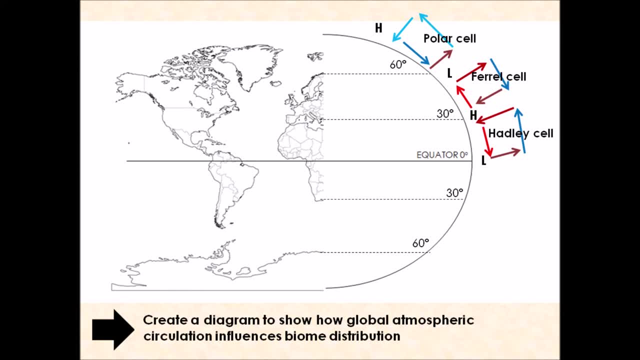 Because the air is descending, it's coming down. At 60 degrees north between your polar cell and your ferrule cell, you've got another area of low pressure- okay, that rising air. And then at your polar cell, right at the north pole, you've got that area of high pressure because the air is 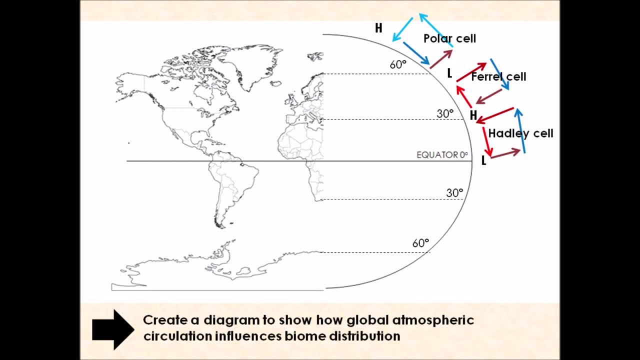 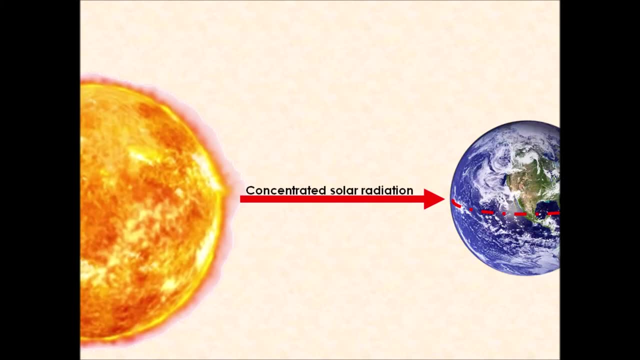 descending and sinking. Now, how does this then relate to biome distribution? Well, if we start off on the equator, we know that the air is rising. So if we look at the equator, we know that the air is rising. So if we look at the equator, we know that on the equator it receives the most intense. 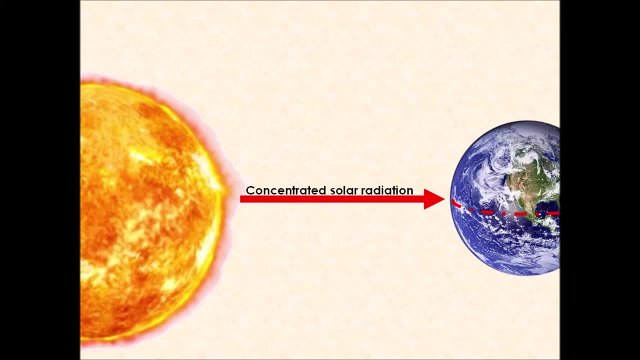 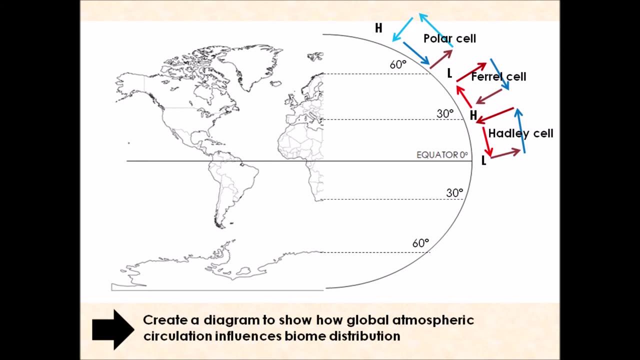 solar radiation and insulation. So, as we have got intense temperatures, this is where you're going to get your tropical rainforests. Tropical rainforests have quite consistent temperature throughout the year. On average, they're about 27, 28 degrees in temperature and there's not much fluctuation. 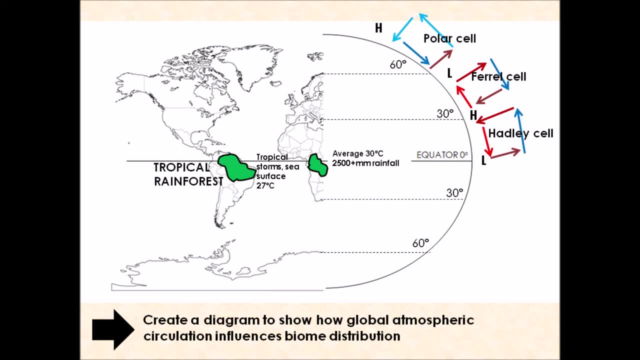 in terms of their annual temperature. Now, because we have a lot of high pressure, we're going to have low pressure areas on the equator And we've got that air rising to form condensation, to form clouds. This is where we would then have high amounts of precipitation. So we know that the 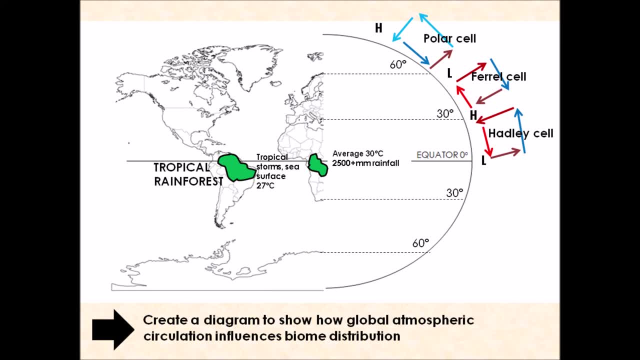 tropical rainforest receives about 2500 millimetres of precipitation a year, if not more. and if you also relate to weather hazards, you will also have on your intertropical convergence zone your warm sea temperatures of about 27 degrees. So this is where you will have tropical storm formation. 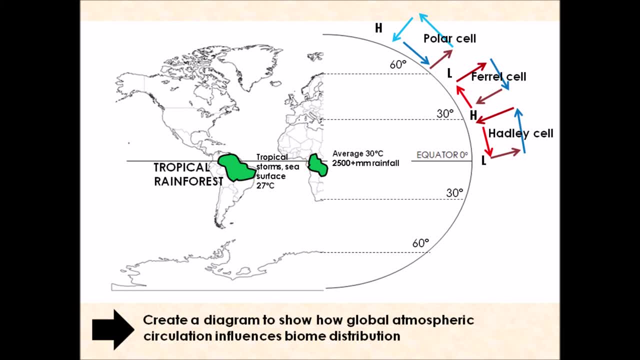 beginning to happen, which then creates your typhoons, your cyclones and your hurricanes. Now, if we start to then move more north, further away from the equator, we're now going to be basically between 30 degrees north and the equator, And this is where we would have some desert. 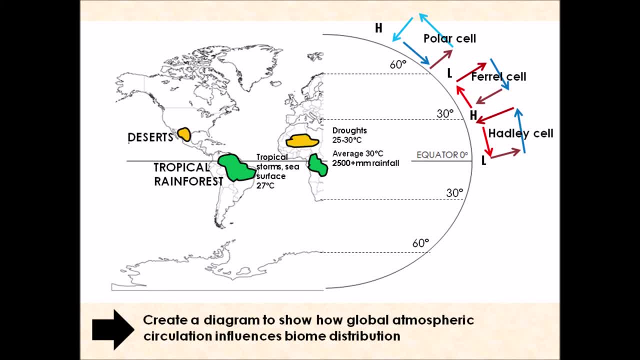 regions. This is very much influenced by the Hadley cell, because we have this convection of air where it's rising at the equator and then it's sinking and starting to descend at 30 degrees north and traveling back towards the equator. So your desert regions would occur in this kind of. 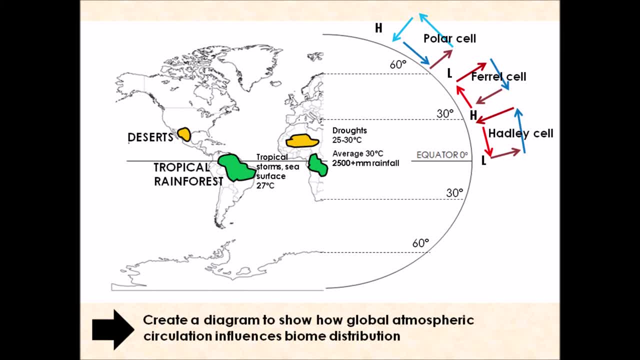 band And deserts obviously can experience temperatures between 25, 30 degrees on average. We have some rainfall, but not as intense, potentially, as your intertropical convergence zone, so on the equator, But this region may experience droughts from time to time as well. Now, moving in a more northerly direction, 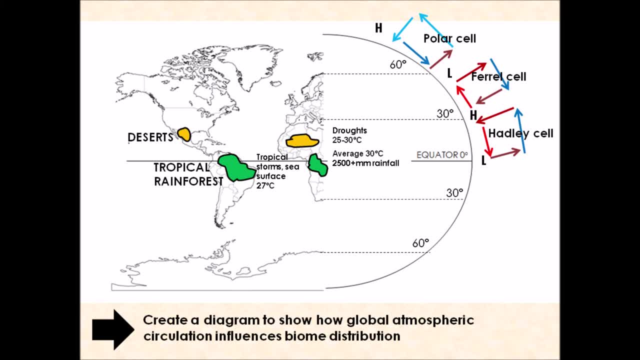 we're now going to be basically where your feral cell then comes into play. So, 30 degrees north you're looking at your Mediterranean type climate, so temperatures between 18 and 30 degrees, And this is where you would start to see a lot of droughts. So you're going to be looking at 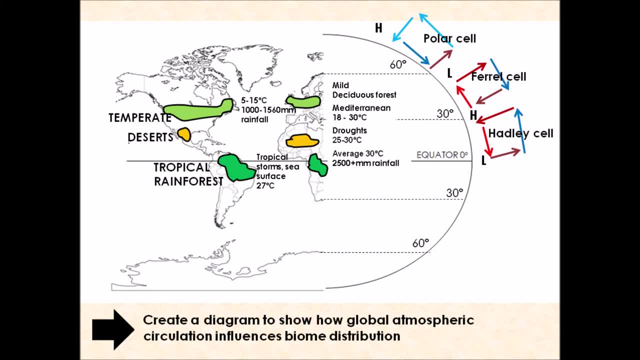 your temperate biomes, so your deciduous forests and your coniferous forests. Temperatures are quite mild and very much can fluctuate at this particular region because, don't forget, this is where we will have that less concentrated amount of solar radiation, So the further we 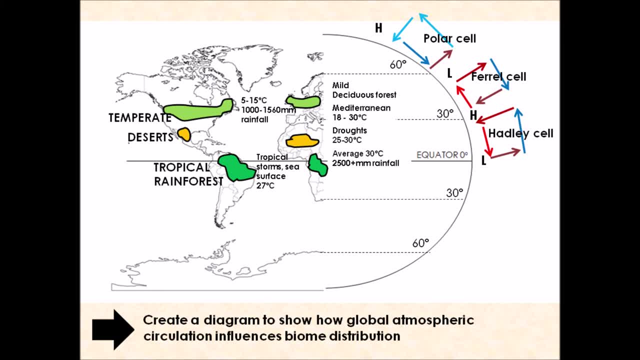 travel away from the equator, the less amount of sunlight that latitude receives. So if we then move towards our polar cell, this is where we're going to see a lot of droughts. So this is where we will experience first of all, on about your 60 degrees north, kind of latitude you're going to. 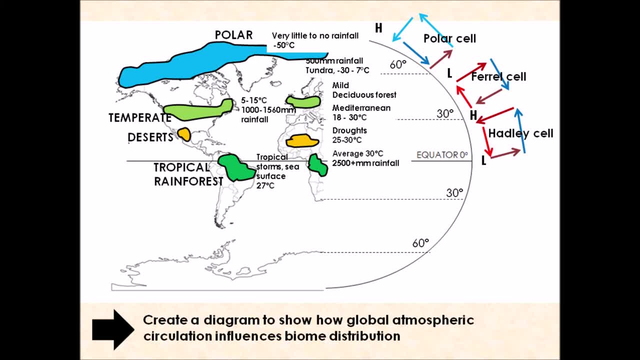 have your tundra biomes ranging from temperatures between minus 30 to 7 degrees, Obviously do receive some rainfall here, some precipitation, because the tundra is located on a low pressure belt, on that 60 degree north kind of location, because we have rising air between our polar and. 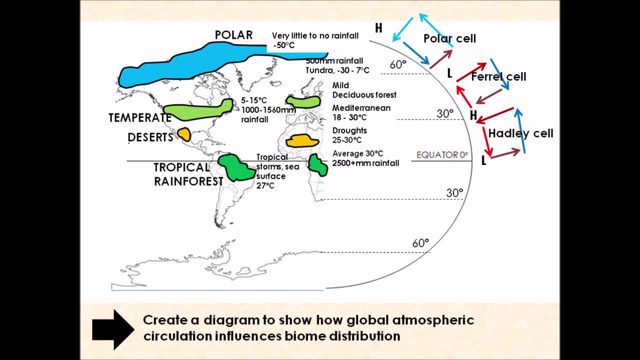 feral cells. But as we travel more towards the North Pole and we get to those higher latitude locations, we are going to experience very little to no precipitation due to the air descending and sinking in those areas of high pressure, And this is where we would have our polar biomes distributed. 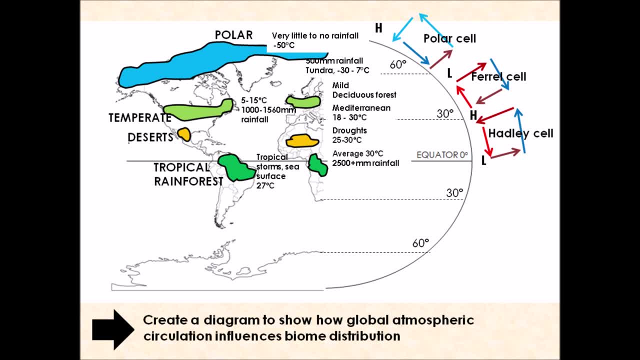 that can reach temperatures up to minus 50 degrees, but they do experience that limited precipitation. Don't forget your pole will receive the least amount of solar radiation and solar insulation, And that is why these particular biomes experience very drastic, very extreme cold temperature conditions. 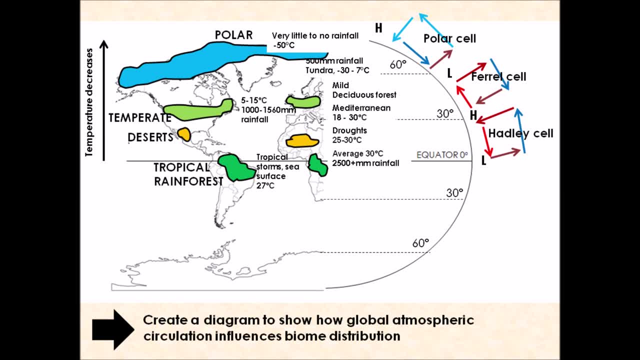 To quickly summarise the diagram then, just on the left hand side, what you should then hopefully say, as we've moved from the equator and your intertropical convergence zone up towards the northern hemisphere, is that linked to latitude and linked to the solar radiation the planet receives. 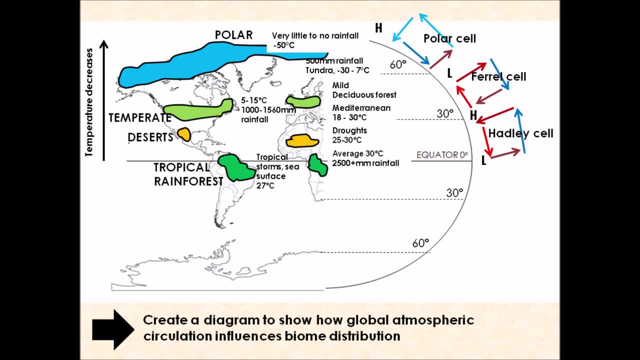 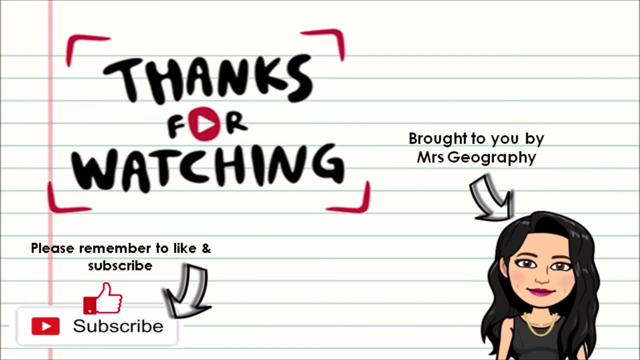 we have that decrease in temperature. So this is basically how global atmospheric circulation and your distance from the equator influences your biome distribution, your weather hazards and your climate zones. So, as always, everyone, I hope you found this video useful. Thank you so. 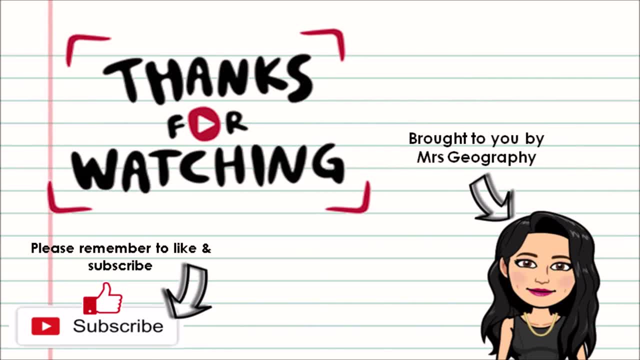 much for watching. Please do like and subscribe and I'll see you in the next video. Bye, And don't forget to subscribe if you are finding them useful and I'll see you next time. 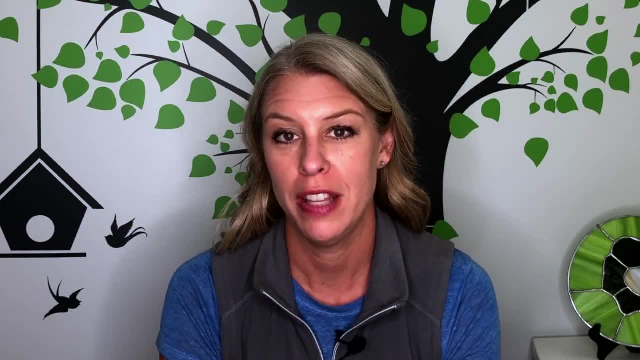 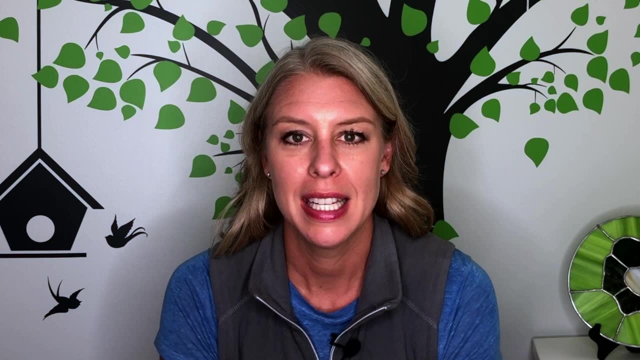 When I was in seventh grade, my friend Amy talked me into joining the cross-country team. At the time it sounded like a great idea. It was an opportunity to stick around after school, get some exercise and be with my friends. It didn't even matter that I was terrible.